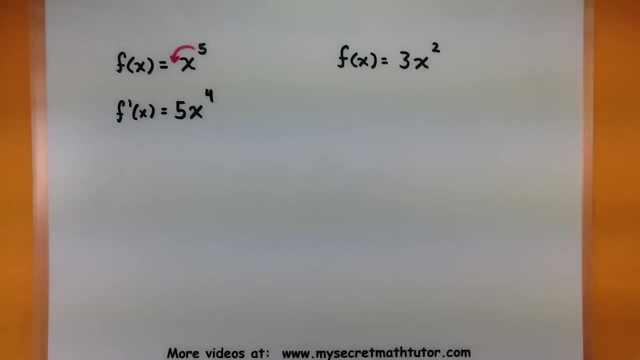 power. Just that simple, All right now. every once in a while you'll come across the function that might have some additional power. So let's say that I have x raised to a number power. So I'm going to take that power, drop it right out front. Now, if these are just numbers, then feel free to. 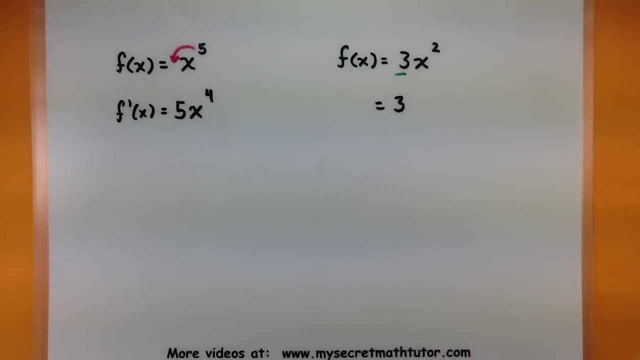 move them So that 3 will still be there, and then apply the rule to the rest of it. So I'm going to take the 2, drop it right out front. So now I have 3 multiplied by 2. There's my x, and now we reduce. 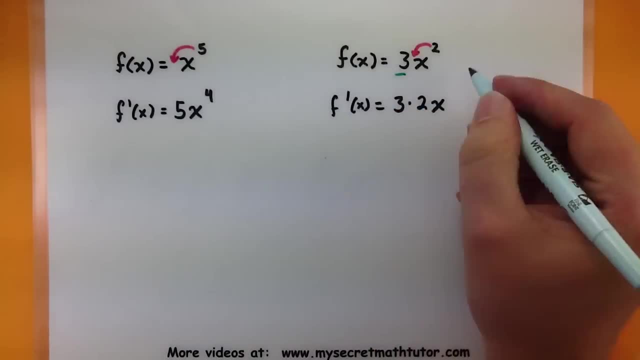 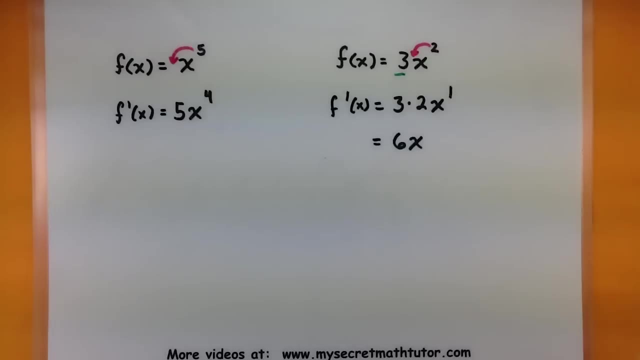 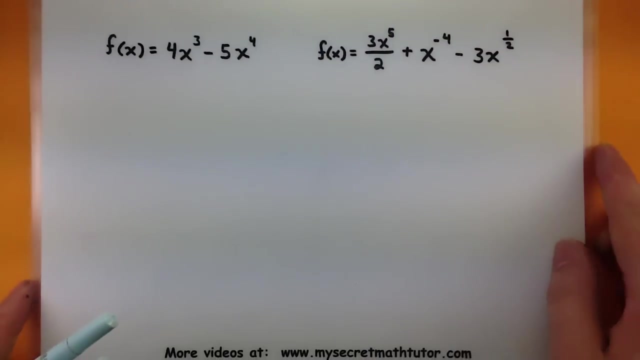 that power by 1.. So 2 minus 1 is 1.. Or this is simply 6x. So as you can see, really powerful rule and it works with all kinds of other powers. Let's check out some more examples and make this a little bit harder. Okay, so in this, 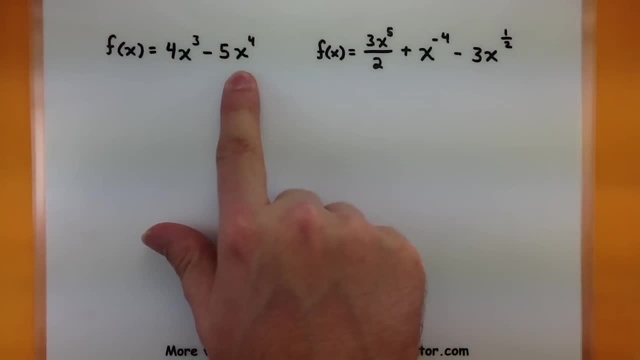 one. you'll notice that I have 4x cubed minus 5x to the fourth. I'm going to apply that power rule to the x cubed and to the x to the fourth. I can do this because they're being connected by plus. 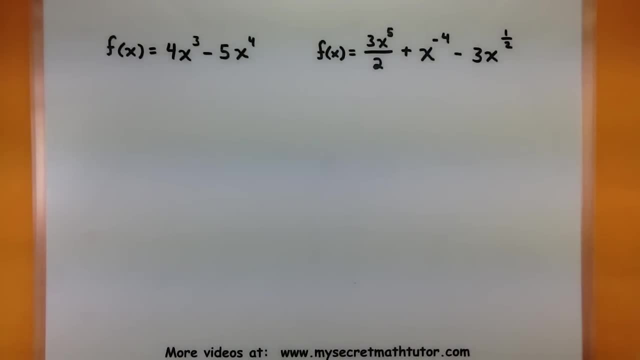 or minus. You can use it in either one of those. So I'm going to take the 2, drop it right out front and see what happens in both situations. All right, let's write out what we got. So f prime of x. 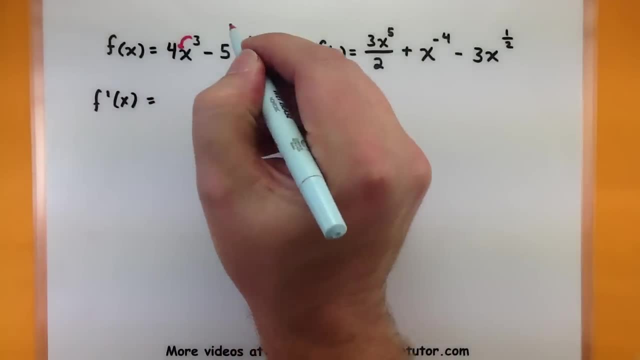 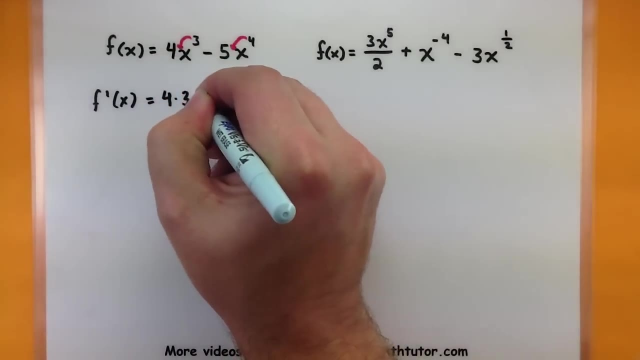 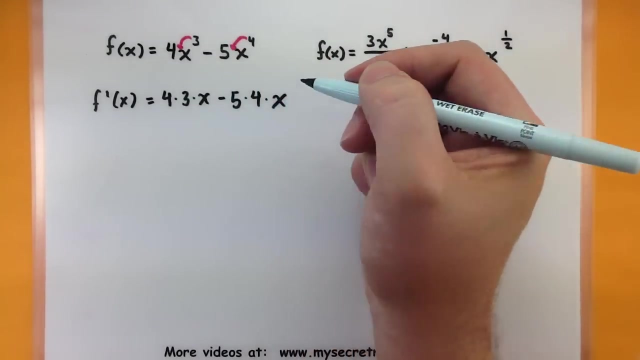 So we're going to drop down the 3. Put that right out front. Drop down the 4.. Bring that right out front. This will give me 4 times 3 times x minus 5 times 4 times x. Now I have to write in the new. 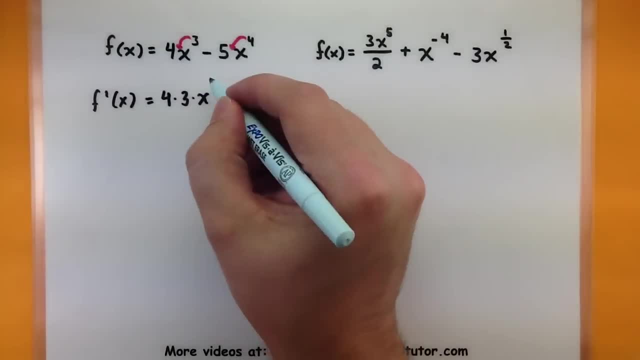 powers. So the 3 gets reduced by 1.. Now it's now a 2.. I have to take the 3 and put it there, So you will see that everything is going from square root to square root. Nobody's going to see a square. 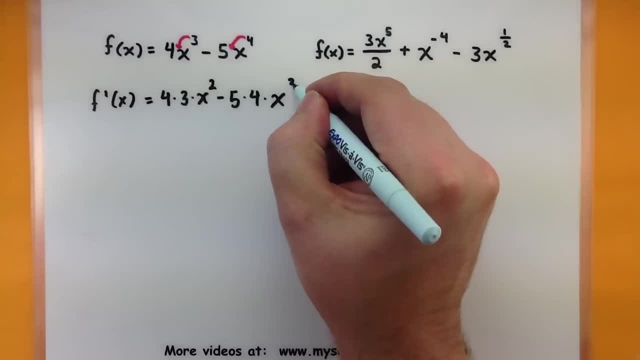 square. All I have to do is divide the power by 3. And there's going to be a power method. So this two, the four, gets reduced by one. it's now a three. Okay, so now we just have a little bit. 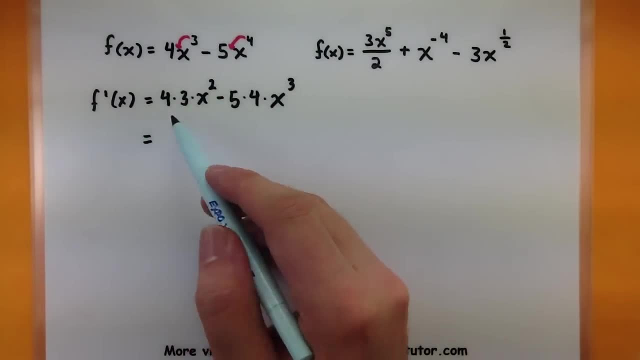 more cleaning up to do and then this one's finished. So four times three would be a 12 x squared. five times four is a 20 x cubed, All right. so one thing that often gets lost with the power rule is: as long as that power is a number that is not zero, you can use it on it.